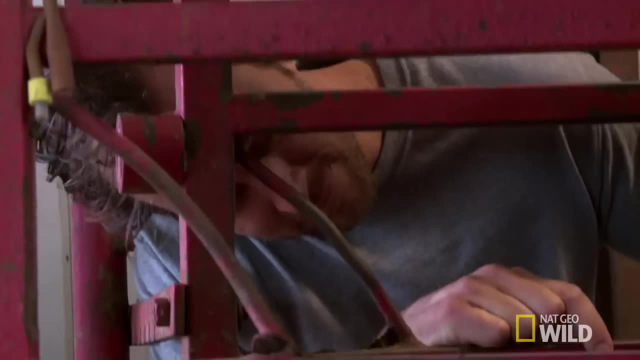 Hold his tail so he won't kick me. Reach underneath And you'll see his testicles there. Oh yeah, I see them. They're pretty hard to miss. So what you want to do is put both of them inside that band. 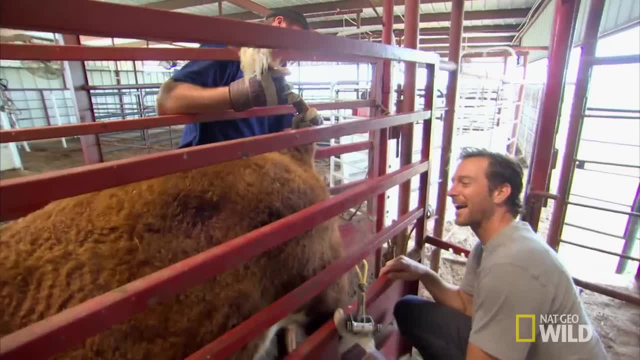 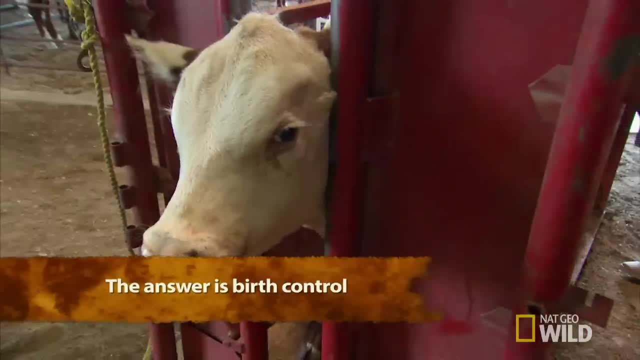 Are we castrating this guy? We are Why, Why, Why. I'm so sorry for you. Oh, Oh man, Why do we need to do this? So you got to get both of them through that little bitty rubber band. 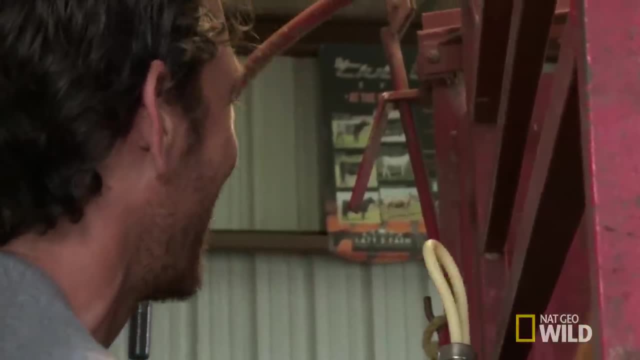 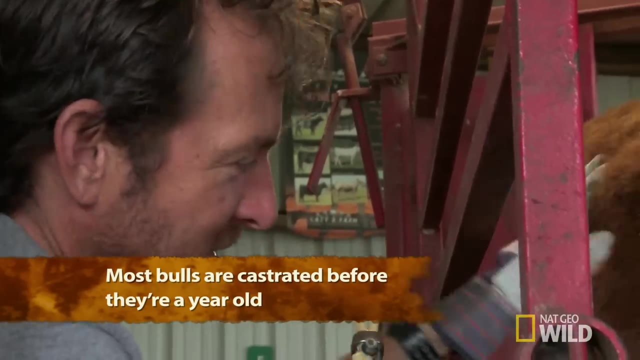 How old? Both of those things In between, this little rubber band. How old is this guy? This guy here? he's seven months old, Seven months. Yeah, I'm sorry, buddy. Yeah, Sorry to do this, So I put this whole thing in here. 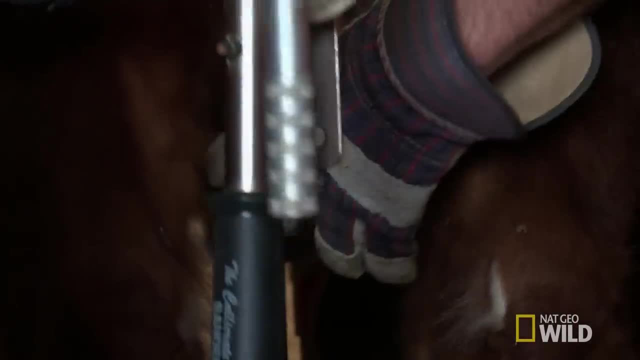 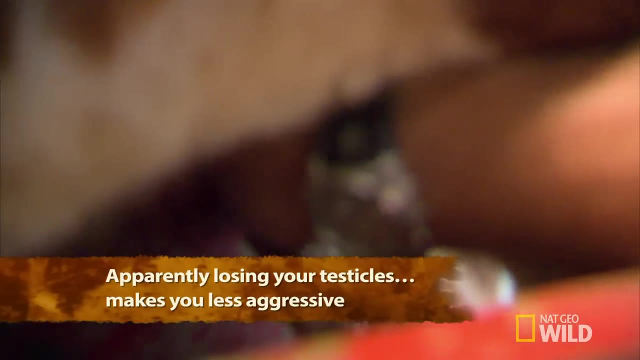 Yep, You're going to grab this with your hand and you're going to have to feed that band. I'll hold this like this. You can do that. Yeah, Oh, I got to feed these through here, right, So this band goes on him. 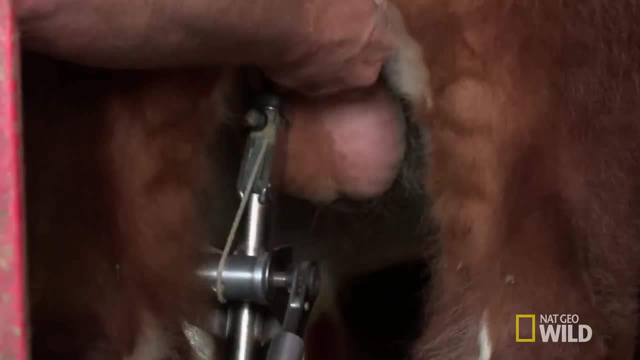 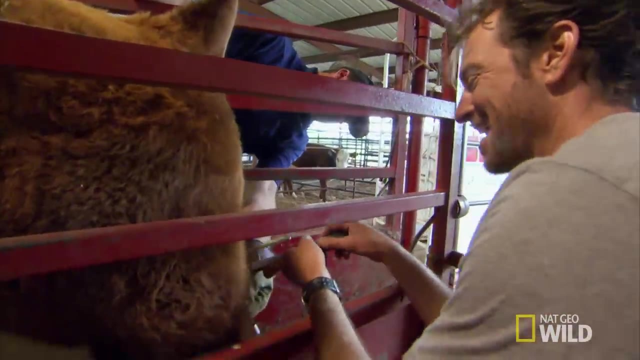 Yep, What's the most painful part? Nothing, Okay, We got it on The first few days. There you go, We got both. Yeah, We got both testicles down Okay. So ratchet that up Okay. 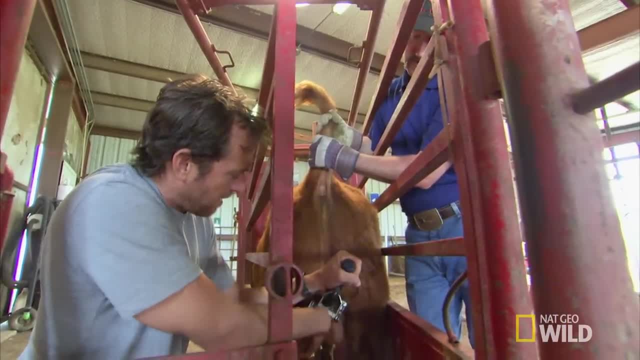 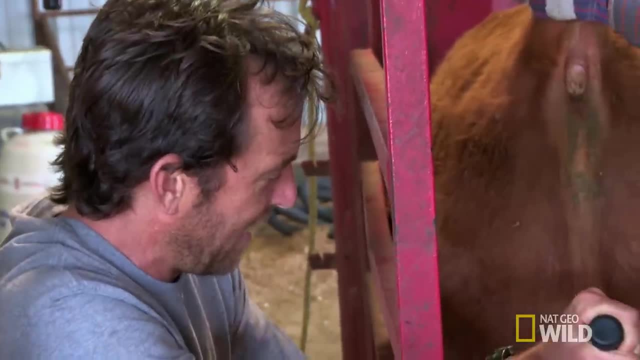 And just keep going, Keep going. Okay, It's going to take quite a bit. Okay, We're going to have to pull up a lot of that rubber band. Just keep going. huh, Yeah, Okay, Oh, the bander. 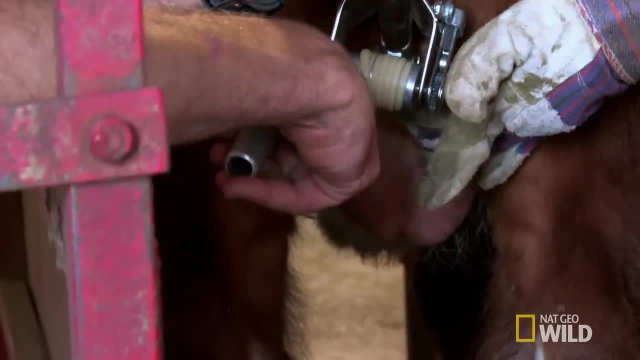 But There you go. Now we're getting close. Okay Yeah, It's getting pretty tight. Oh yeah, We're getting tight. Okay, Now, what you have to do is pull up on this. Pull up on this. 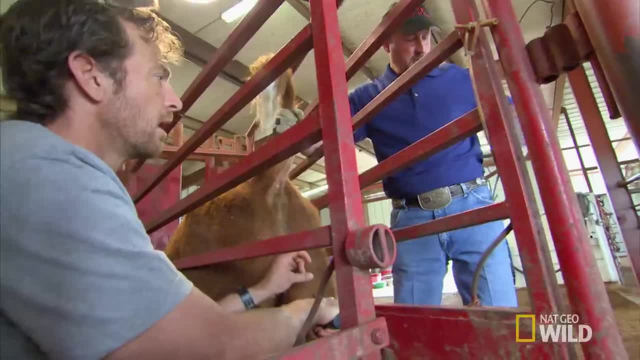 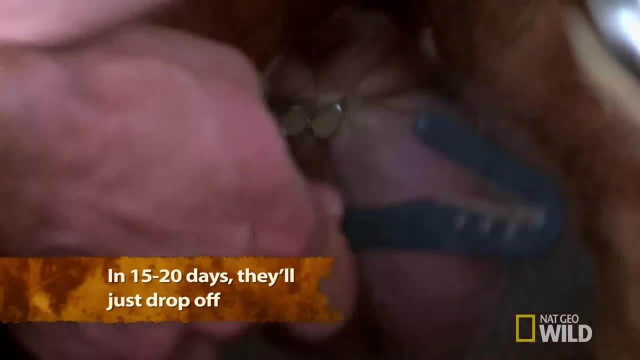 Uh-huh, Uh-huh, There you go, Like that, Perfect, Then you have to take your cutter here, Okay, And you're going to just cut it across. Okay, There we go, That's it. I mean, surprisingly, that seems pretty painless. 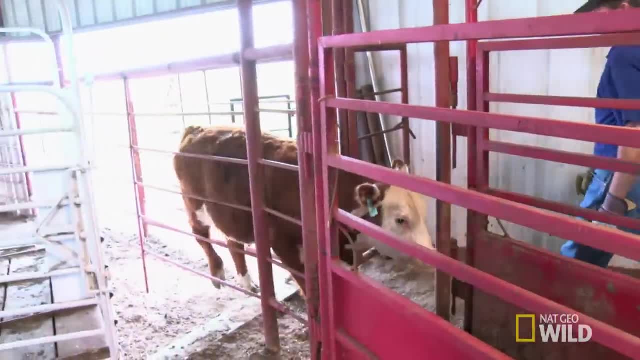 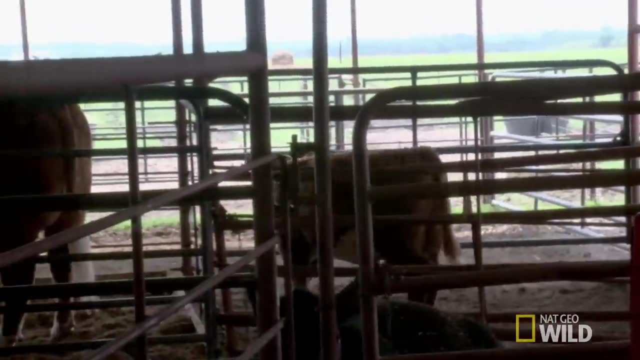 This is the best way to do it. It's the best way. Sorry bud, Sorry 133.. We did it. Let's move on. We'll move on to the next one. 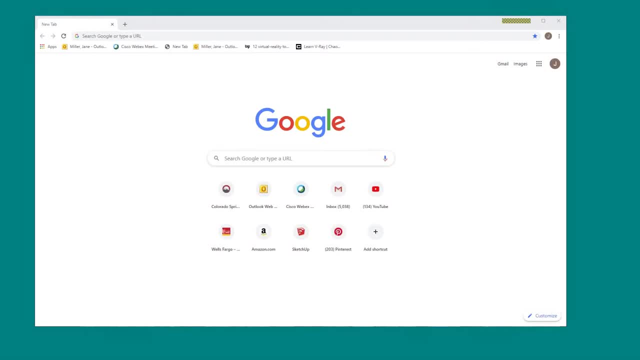 Okay, this is a really fast tutorial on how to get RGB values for specific paint colors. So what we're going to do is we're going to look for Sherwin-Williams- Oops, there is Sherwin-Williams. All right, and here we go. Add comes up.